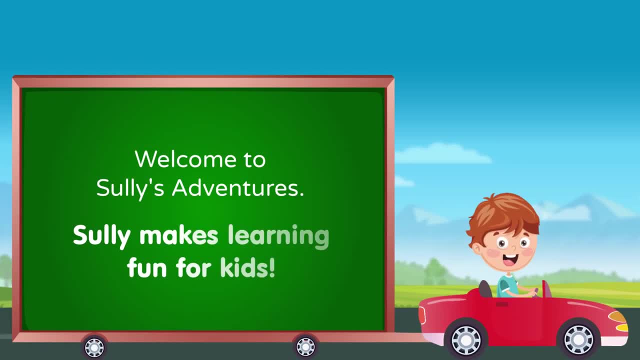 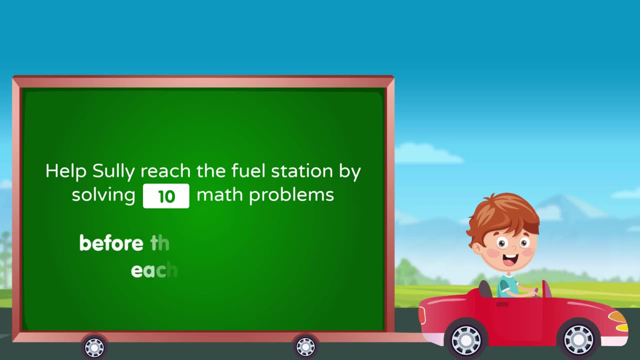 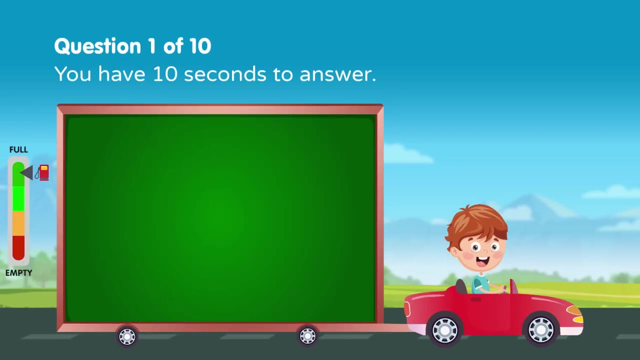 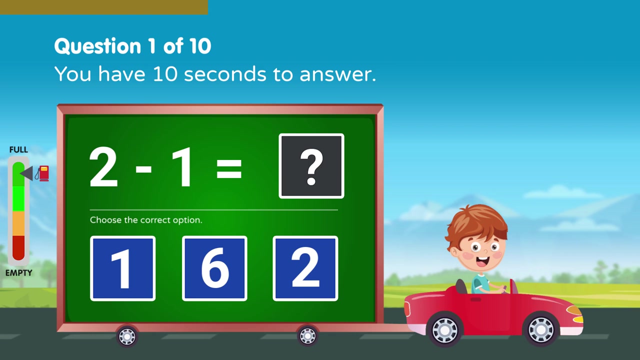 Welcome to Sully's Adventures. Sully makes learning fun for kids. Help Sully reach the fuel station by solving 10 math problems before the timer ends on each question. Solve the following: you have 10 seconds to answer. Solve the following: you have 10 seconds to answer. 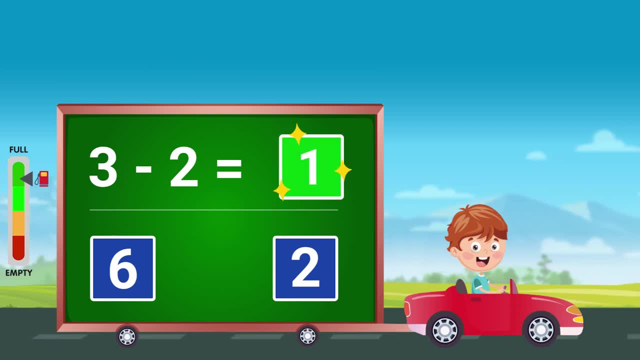 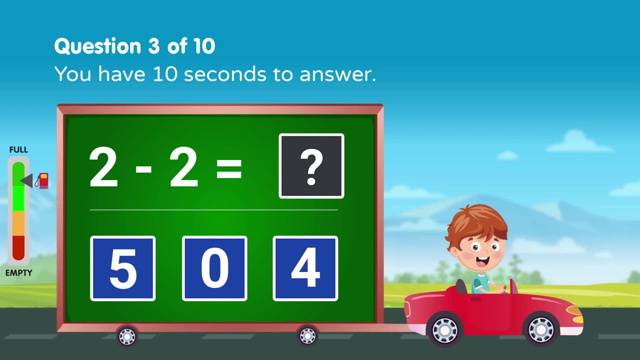 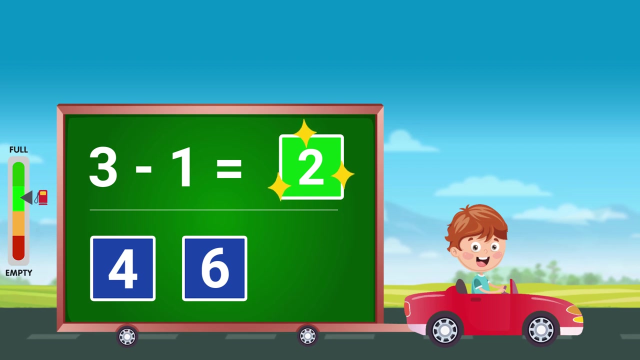 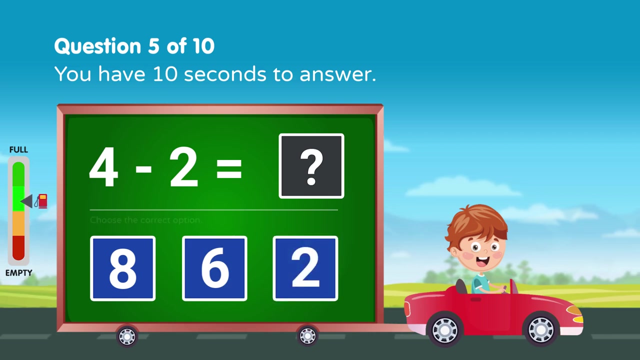 Solve the following: you have 10 seconds to answer. Good job. Solve the following: you have 10 seconds to answer. Good job. Solve the following: you have 10 seconds to answer. Solve the following: you have 10 seconds to answer: 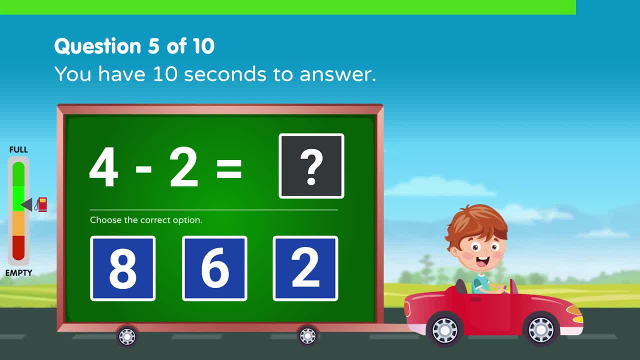 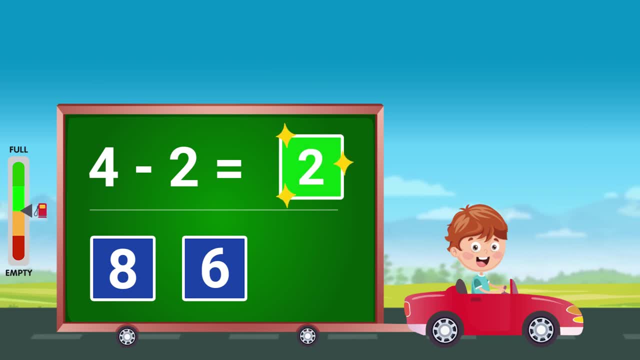 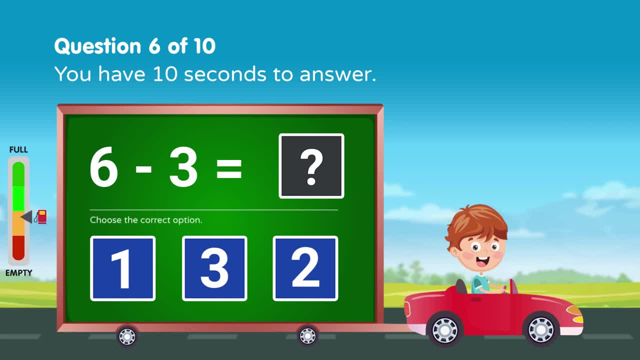 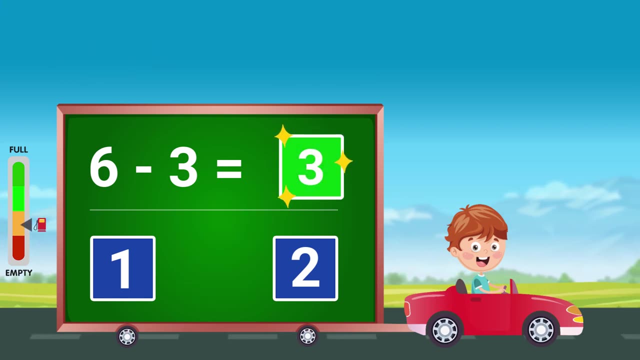 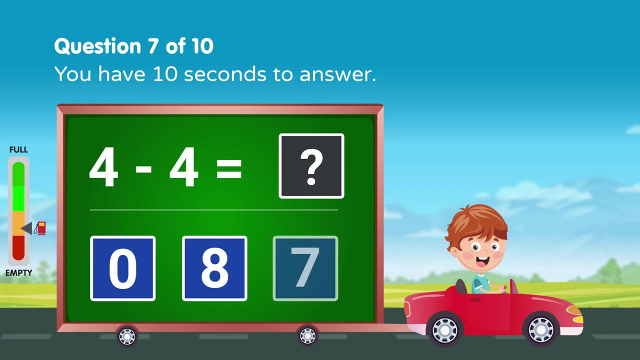